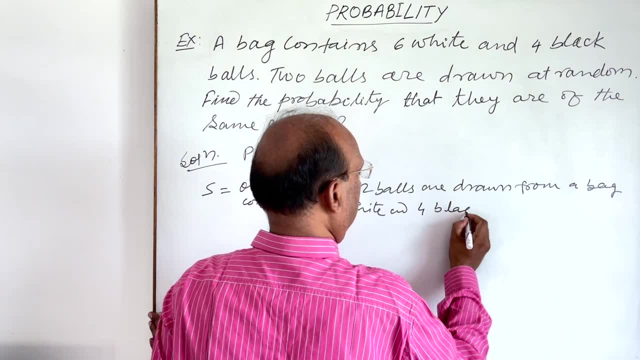 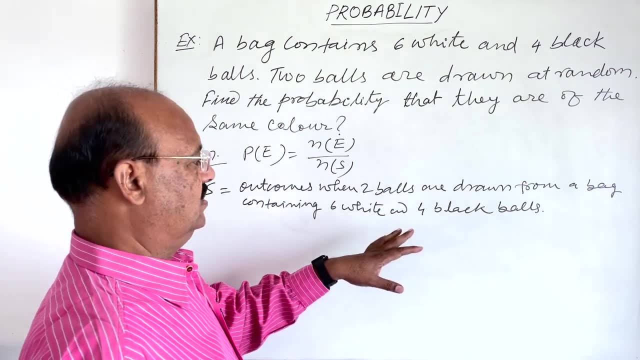 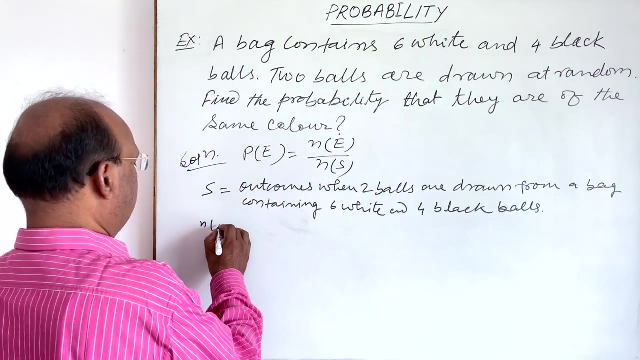 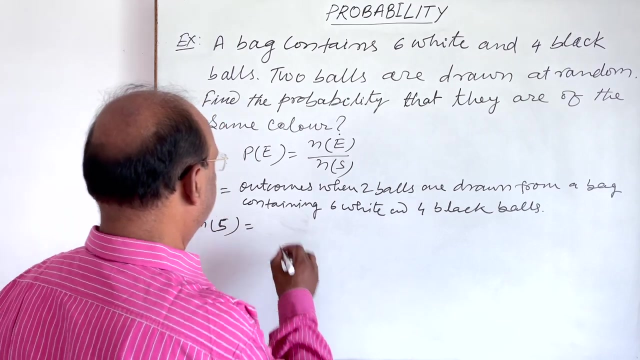 Here. question is: a bag contains six white and four black balls. Two balls are drawn at random. Find the probability that they are of the same color. So, as we have discussed in the previous videos also, that probability of any event is equal to n. 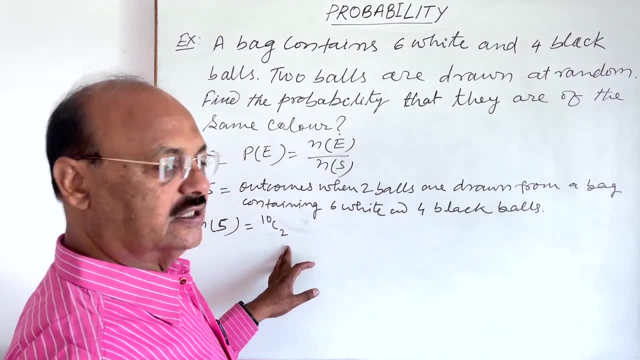 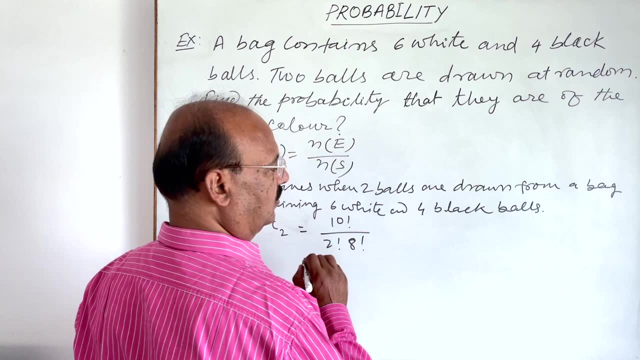 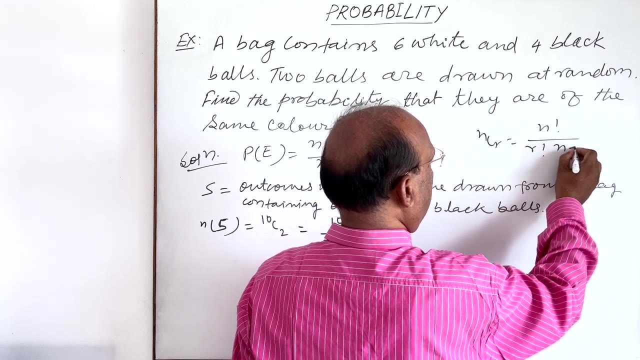 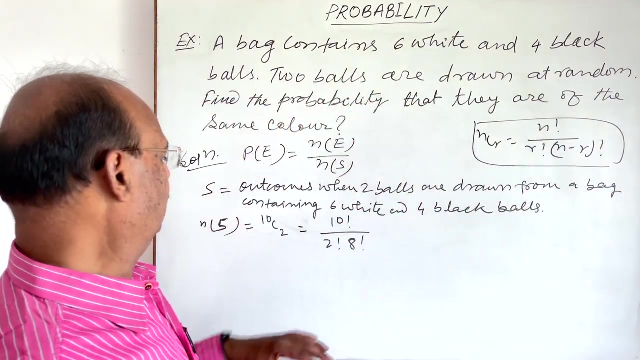 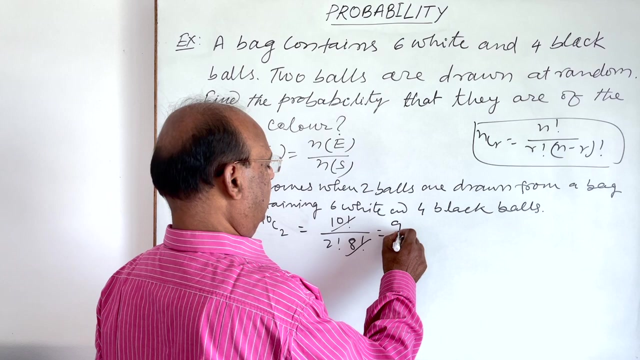 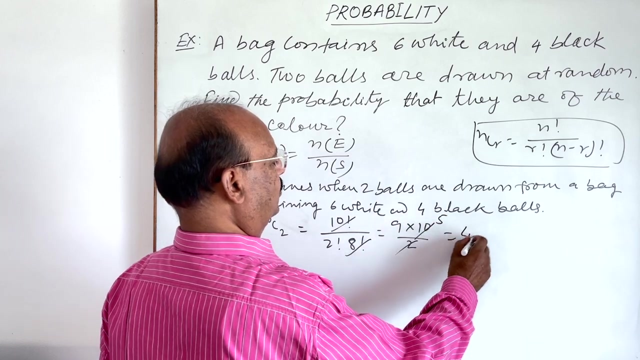 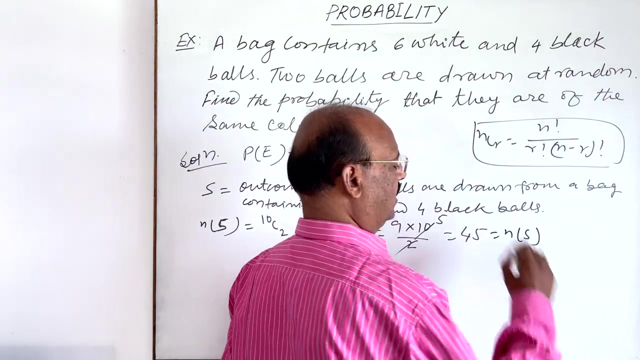 So let us see a very important question from the topic probability Here. question is: a bag contains six white and four black balls. Two balls are drawn at random. Find the probability of any event is equal to n. So numerator will be 9 into 10 and two factorial means 1 into 2, that is 2.. Two 5s are 10.. This is equal to 45.. So this is the value of ns. This we are getting here. Now we have to find out the value of ne. 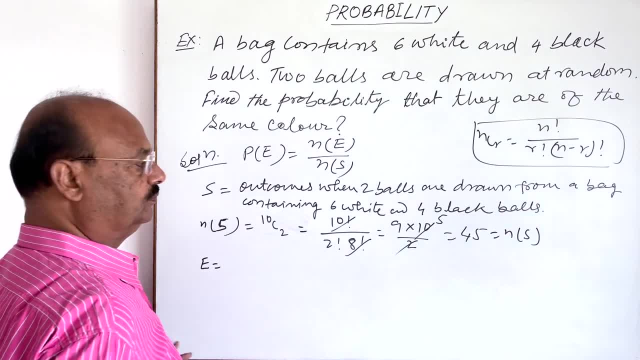 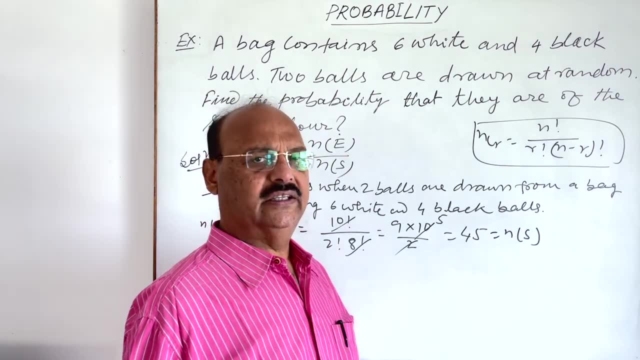 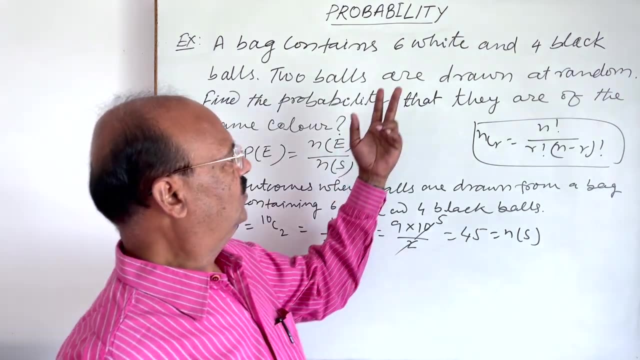 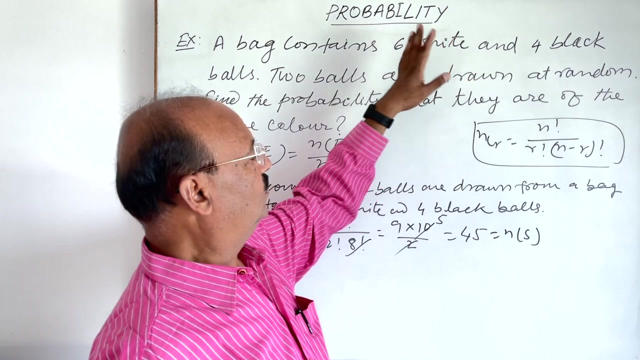 So here, what is the event? e There are two possibilities or two designs. There are two desired cases, Two favorable cases. is here Two balls drawn are from six white balls or two balls are from four black balls. So two balls from six white balls and two balls from four black balls. 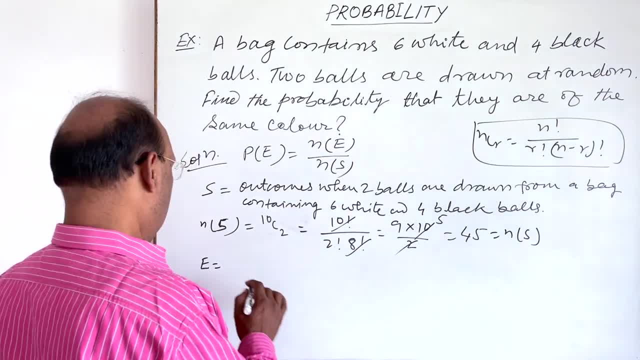 I mean event is a set which consists of favorable event. So we need to find out the probability of any event. So let us see a very important question from the topic probability Here. question is: a bag contains six white and four black balls. Two balls are drawn at random. Find the probability of any event is equal to n. 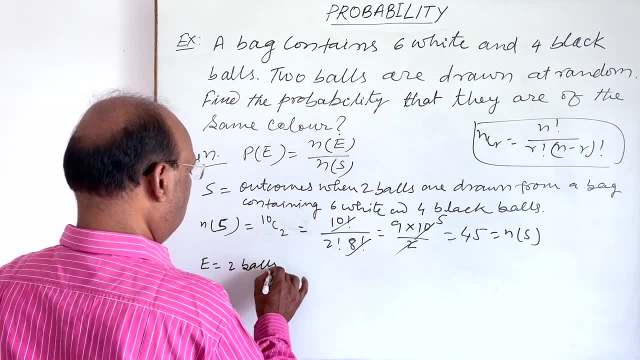 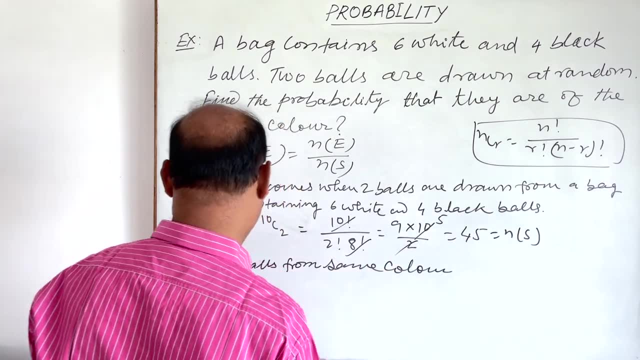 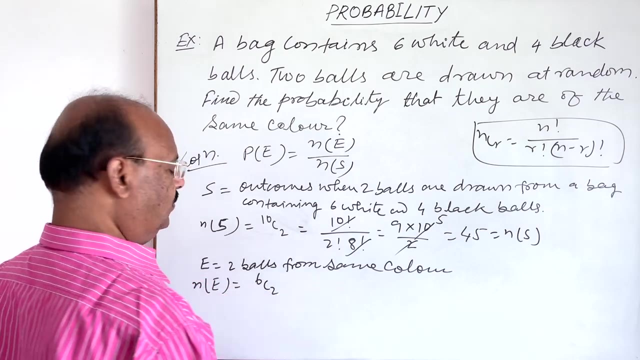 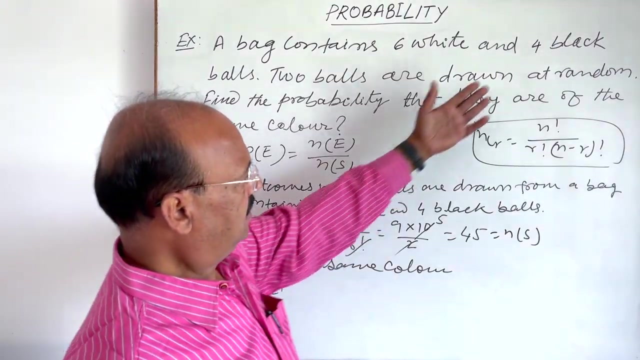 We need here two balls from same color. This is our favorable event. So we can calculate here: ne is equal to: there are six white balls, So 6c2, since we are drawing two balls, And plus again same color is black. So we are getting two balls from black, So that is 4c2..